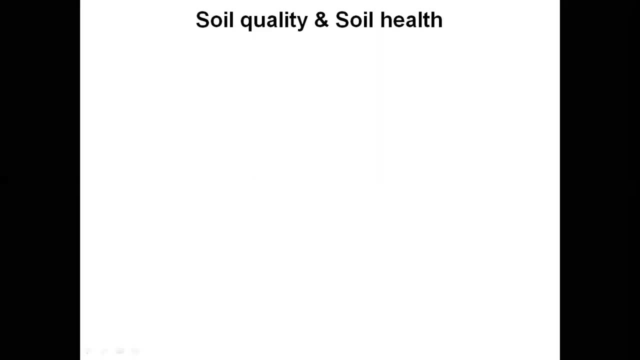 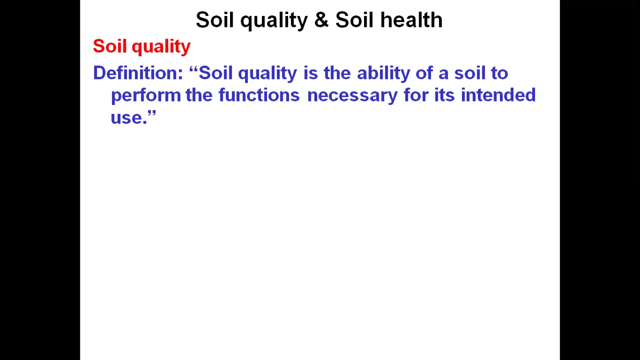 The next topic is the soil quality and soil health. Soil quality is the ability of the soil to perform the functions necessary for intended use. Whatever the ability of the soil to perform the functions necessary for its intended use is known as the soil quality. For example, if we are using this soil for the agriculture purpose, then that soil should have the ability to give the produce from that soil so that it will be used for the agriculture purpose. 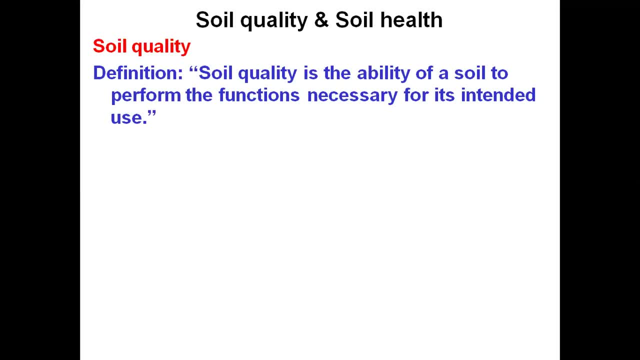 Or another purpose is, whatever the intended use of that soil which is carried out and the ability of that soil is said to be the soil quality, Or the soil quality is the capacity of the soil to function within the ecosystem and land use boundaries, to sustain the productivity, maintain environmental quality and promote the plant and animal health. 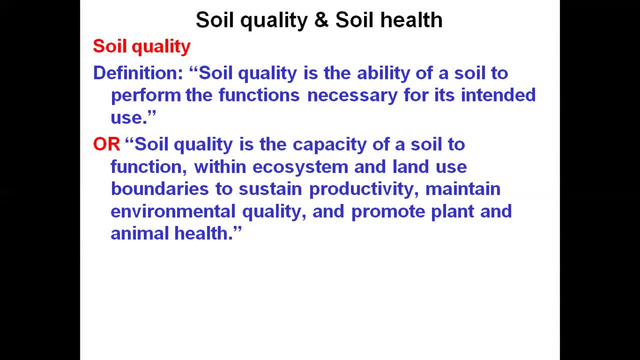 Whatever the capacity of the soil to function within the ecosystem and land use boundaries, to sustain the soil productivity, maintain environmental quality, promote plant and animal health, is known as the soil quality. is known as the soil quality, While soil health is the continued capacity of the soil. 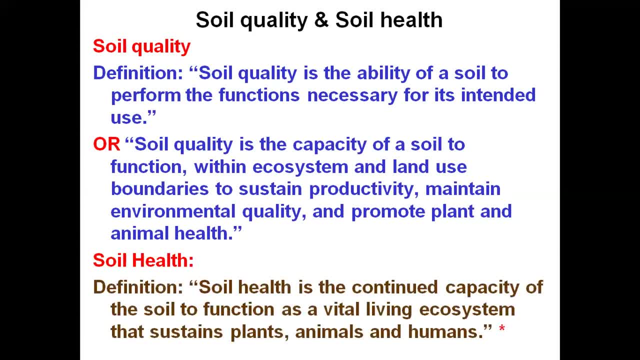 to function as a vital living ecosystem that sustains the plants, animals as well as the humans. Soil quality is nothing but the ability of the soil to perform the functions which are necessary for its intended use, while soil health is the continued capacity of the soil. 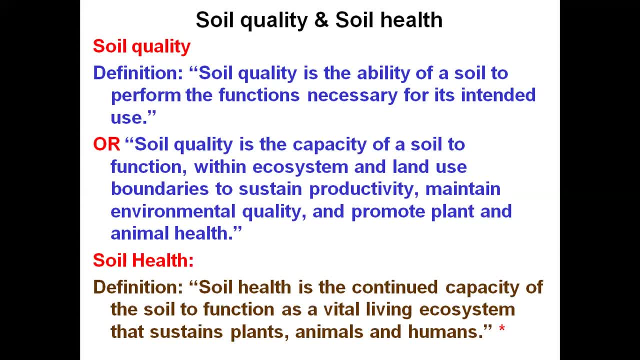 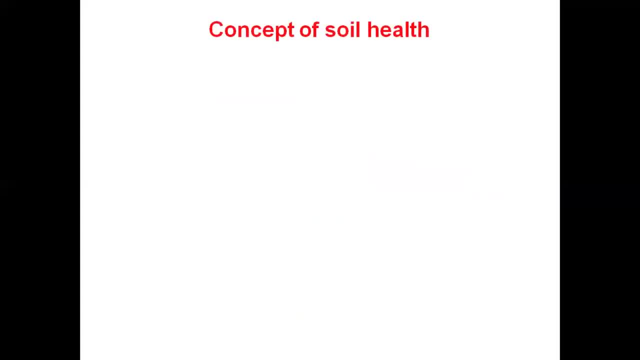 to function as a vital living ecosystem which will sustain the plants, animals and humans. We will see the concept of the soil health In general, soil health and soil quality are considered as synonymous terms, But this soil quality includes both the inherent as well as the dynamic quality. 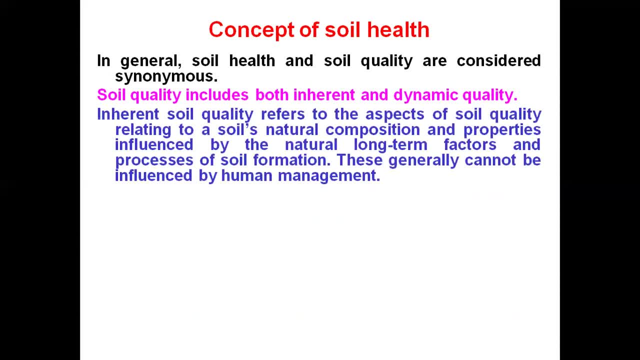 Inherent soil quality refers to the asperity, the aspect of the soil quality relating to the soil's natural composition and properties, influenced by the natural long-term factors and processes of the soil formation. These generally cannot be influenced by the human management, Whatever the soil's natural composition and properties. 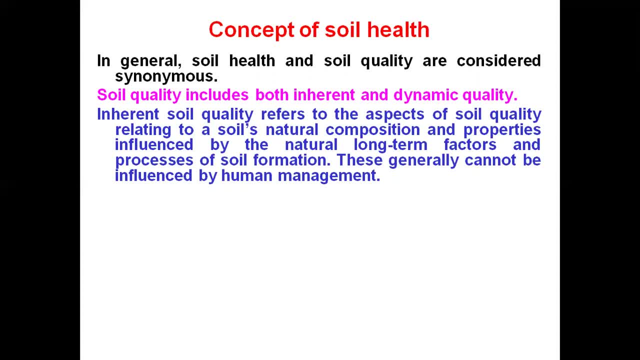 which are influenced by the natural long-term factors and processes of the soil formation but cannot be influenced by the human management, are the inherent soil qualities, while dynamic soil qualities are the equivalent to the soil. health refers to the soil properties which can be changed as a result of soil use and management. 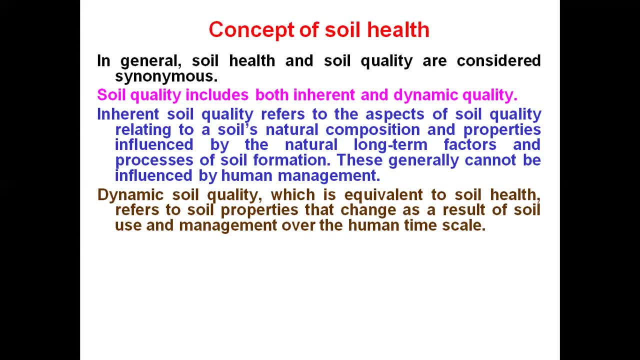 for the human time scale or the use which is carried out by human, whatever the properties of the soils which can be changed due to the use of the soil or the management of the soil which is carried out by the human being, that is known as the dynamic soil quality, soil health. 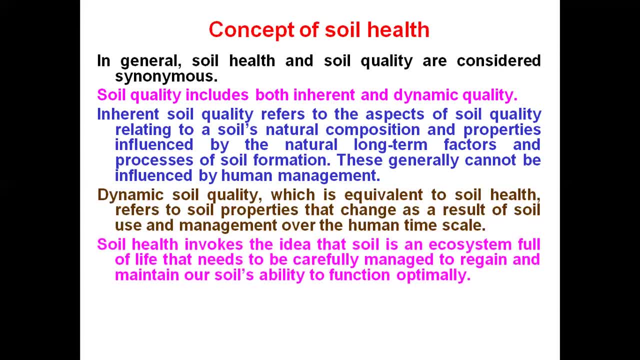 involves the idea that soil is an ecosystem full of life that needs to be carefully managed to regain and maintain our soils ability to function optimal. the term soil health has been generally preferred by the farmers, while the scientists they have generally preferred the term soil quality, because this related with the soil health, soil properties. 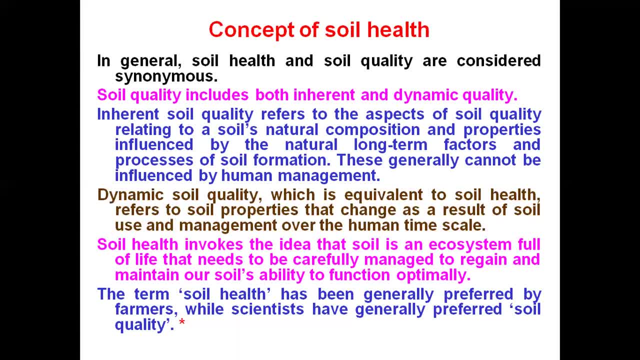 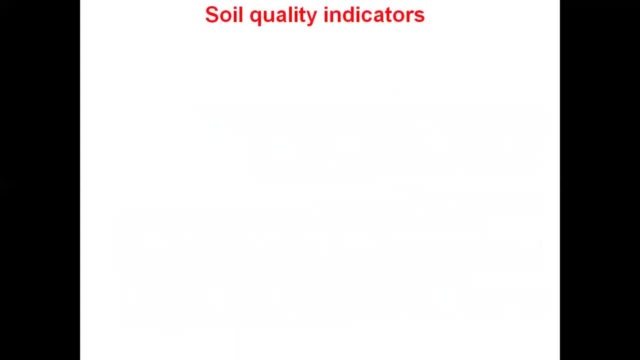 and this will be affected by the use of the land or the management practices. then we will see what are the different types of soil health and what are the different types of soil properties and different soil quality indicators. this soil quality indicators are used to evaluate how well soil will. 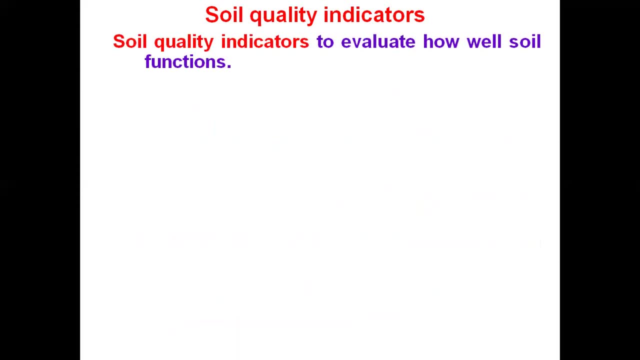 give the function. how this soil will functions, and this evaluation of the soil functions will be indicated by the soil quality indicators. ideal soil indicators should be correlate with the ecosystem, integrate soil physical, chemical, biological properties, as well as the processes, be accessible to the many users, be sensitive to the management and climate. 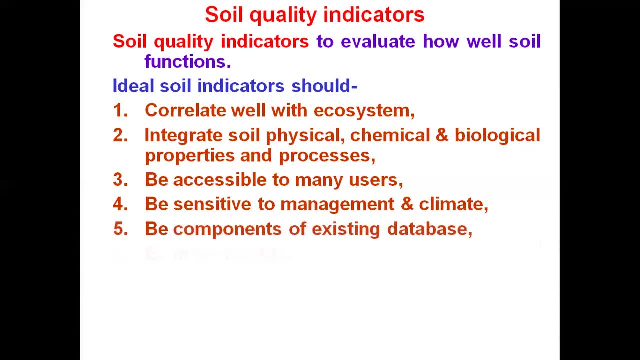 be component of existing database and be interpretable. this ideal soil indicators should be integrated into humanity, integrated into the climate and make plasma plant environment strain dependence community property��. therefore, it is 싸이러 뱇히는 is important to understand that the nature of the plant and how they behave. 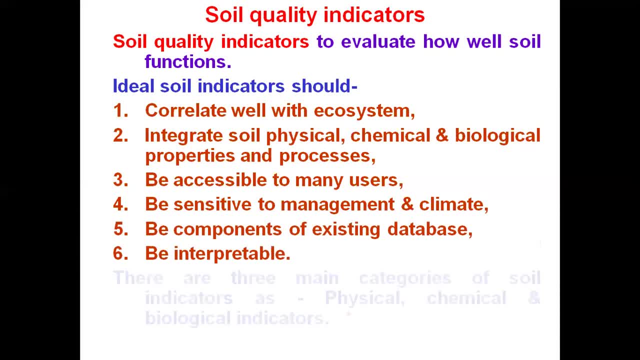 and for being on heat. therefore, you cannot promote and 어딘가요 use this as a brake, light and stress activity, as a machine, etc. andstyle, etc. etc. after providing a well planned and systematic workflow for the development of scientists of the soil. 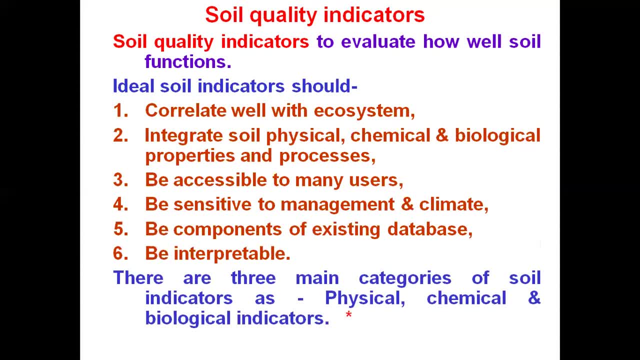 is that花 jim and stuff out. you like this particular scenario, so try to love simple tips from the food areas with allistirds. is that afect medical biomass or other malicious foreign solutions such as mutual risk stakeholders and sexello or illegal services? Eliza İnsport is not material essential to humanыл. 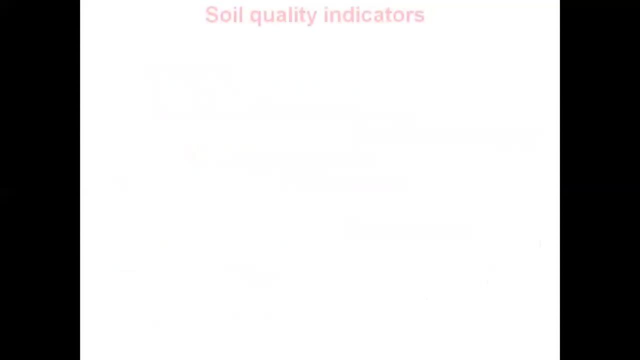 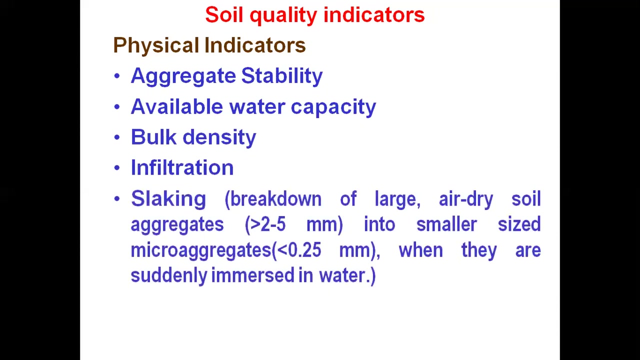 biological indicators. we will see the soil quality indicators first of all, the physical indicators. first important soil physical indicator is the aggregate stability. another one is the available water capacity, bulk density, infiltration and slaking, that is, breaking of the large air dry soil aggregate greater than 2.5 millimeter into smaller size microaggress less than 0.25 millimeter. 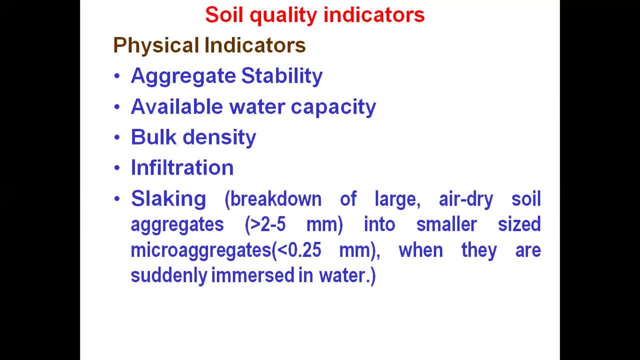 when they are suddenly immersed in the water. if we see the physical soil quality indicators, there may be the aggregate stability available water capacity in the soil quality indicators. we will see the physical soil quality indicators. there may be the aggregate stability available water capacity in the soil. density of the same infiltration of the soil are slacking of that soil. 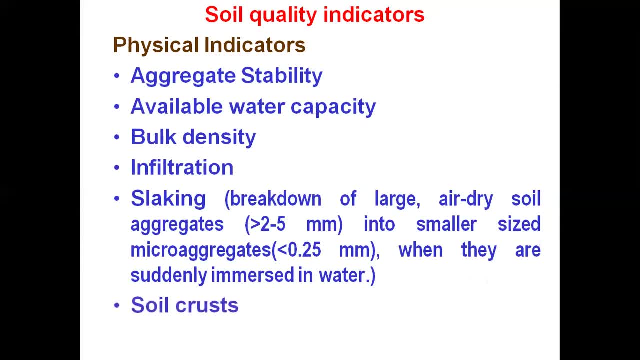 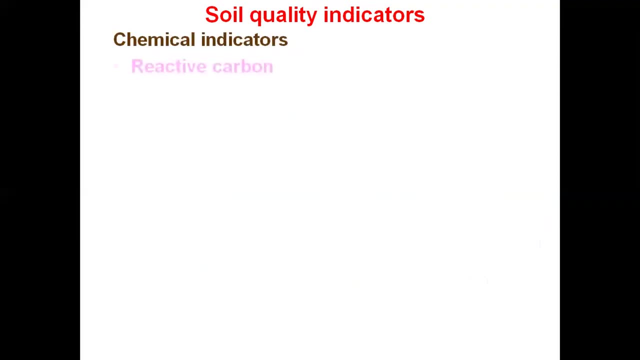 deeper sea nano. There may be: the reactive carbon present in the soil, electrical conductivity of the soil, soil nitrate present in that soil, pH of the soil. These four are the chemical indicators of the soil quality, in that reactive carbon, electrical conductivity of soil, soil nitrate and pH of the soil are the chemical indicators. 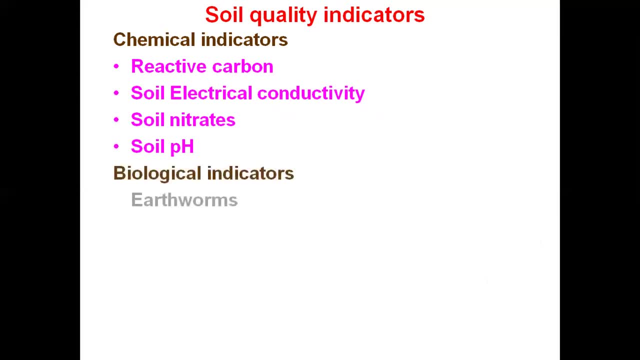 And the biological indicators are the earthworms particulate organic matter which is present in that soil, potentially mineralizable nitrogen content of the soil, various kinds of the soil, enzymes, soil respiration and total organic carbon content of the soil. These earthworms particulate organic matter. 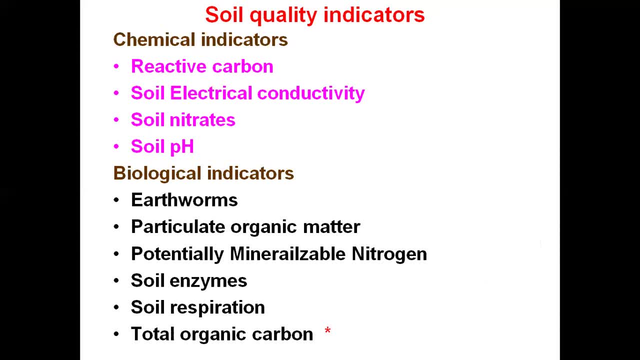 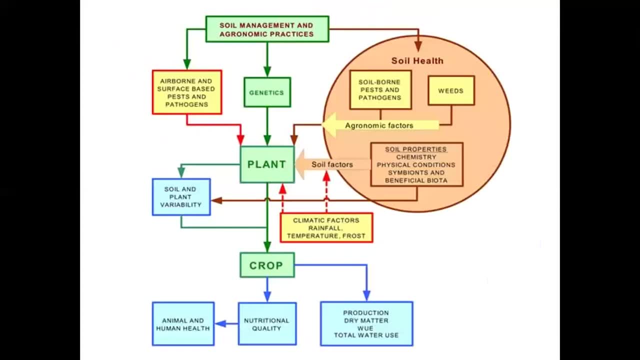 These earthworms. particulate organic matter, Potentially mineralizable nitrogen, soil enzymes, soil respiration, total organic carbon are the biological soil indicators. This soil health and how it is related with the crops, plants, genetics and how these management practices these are carried out. these are shown in these photographs. 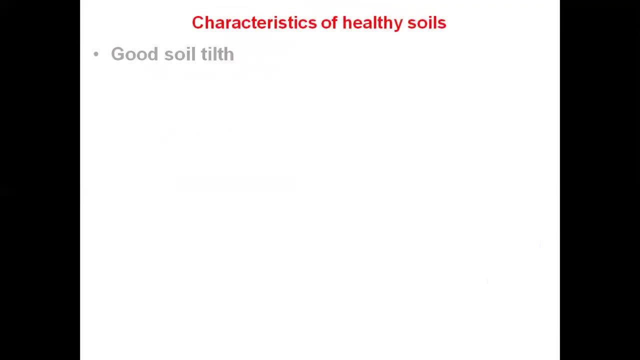 We will see the characteristics of the healthy soils. These healthy soils should have the good soil till- already you have learned the term soil till- and these healthy soils should have the good soil till sufficient depth, good water storage as well as good drainage condition. sufficient supply of the nutrients, but not excess of the nutrients. 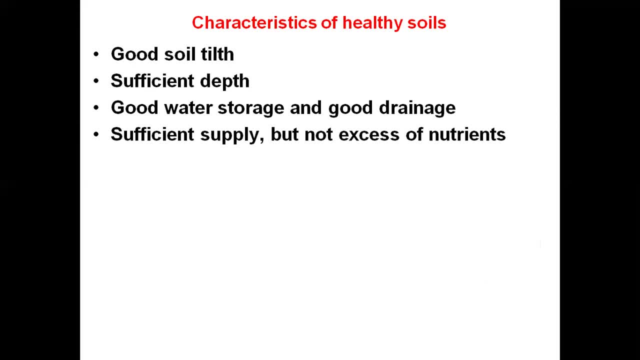 Otherwise it will show the toxicity symbols. Otherwise it will show the toxicity symbols And hence this healthy soil should have sufficient supply of nutrients. Small population of the plants: as there will be the smaller plant population, it will grow healthy Pathogens and insect pest. less population, as these pathogens and insects are reduced. 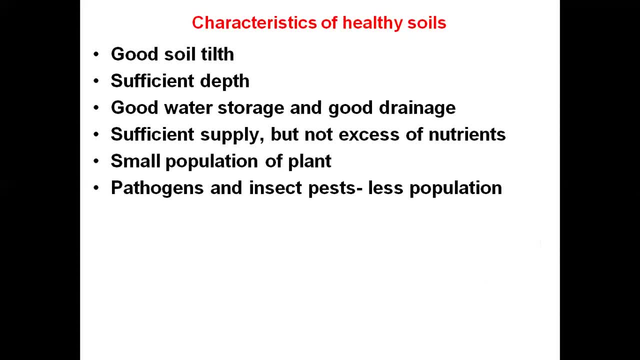 Next we will discuss the pathways on crops. Next we will discuss the pathways on crops of the soil. it reduces the growth of the plants. hence there should be the less population of these pathogens and insect pest, large population of the beneficial organisms so that it will 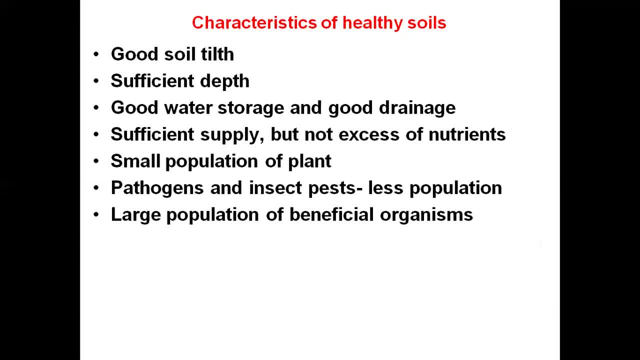 help to give the healthy growth of the plants, which will help to increase the productivity of the soil. low weed pressure: as we know, these weeds are utilizing the all resources which are applied for the crops- water, nutrients. these are used by these weeds, which are not good for the healthy growth of the crops. hence there should be the low weed pressure few.